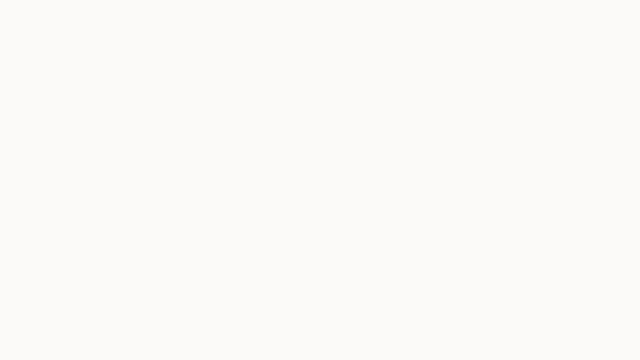 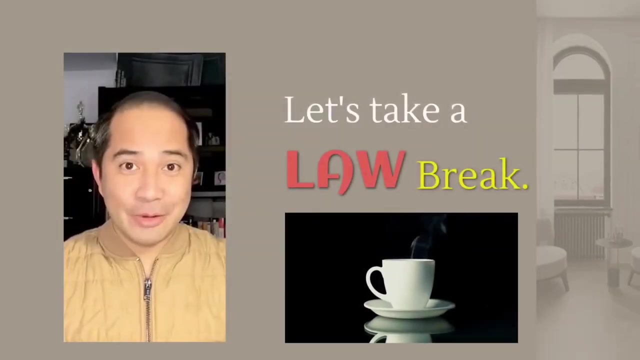 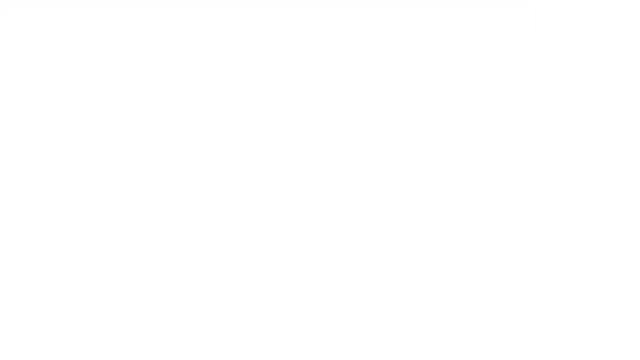 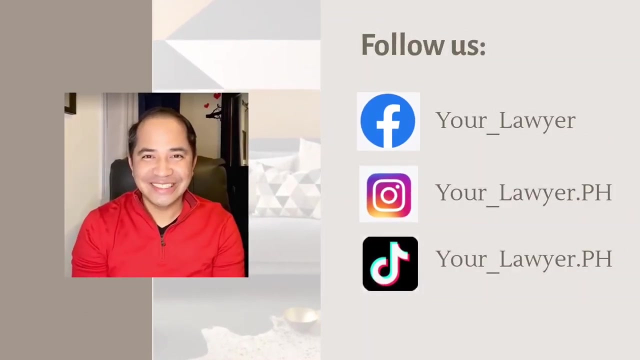 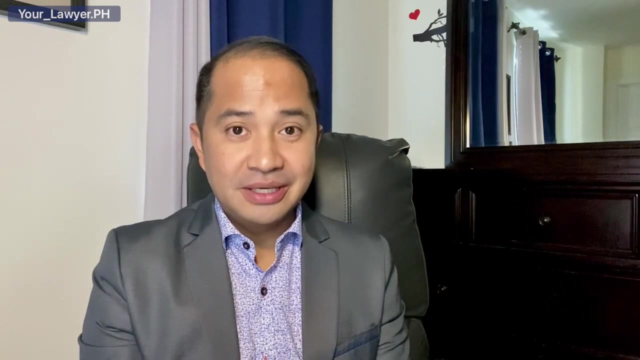 the past. Let's talk about that after this. Hello everyone, how are you? I hope that everyone is doing well, fine and good. If you are new to this channel and you think that this channel can be of help in providing you with useful information, please feel free to subscribe to this channel and don't forget. 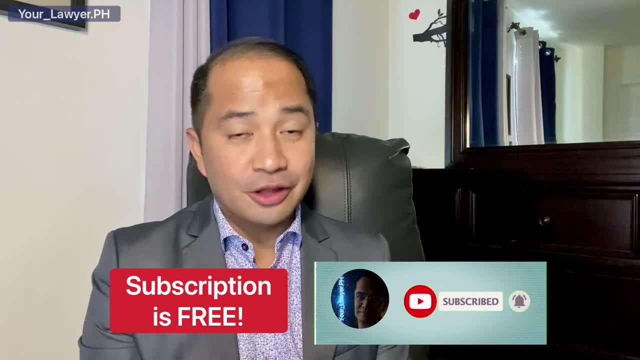 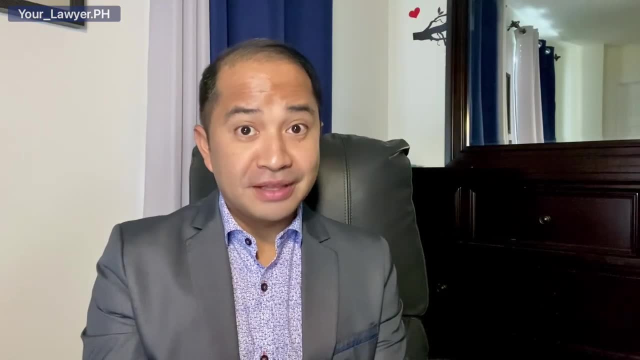 to hit that notification bell icon so that you will get notified of our future videos. Maraming salamat po. Before, kung kinakailangan mo ang isang Philippine document na gagamitin mo abroad, whether for business, for work or for education sa ibang. 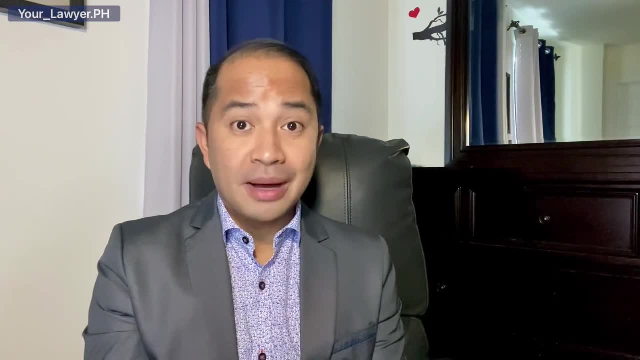 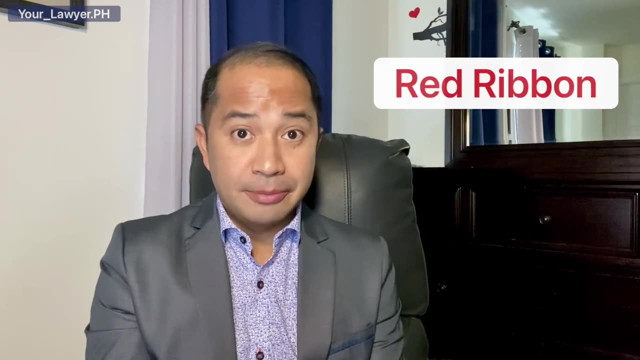 bansa. napakahaba po ng proseso upang maipa-authenticate ang dokumento na to Tinatawag po ang authentication requirement na to na Red Ribbon. Medyo matagal po umahaba po ang proseso ng Red Ribbon dahil. 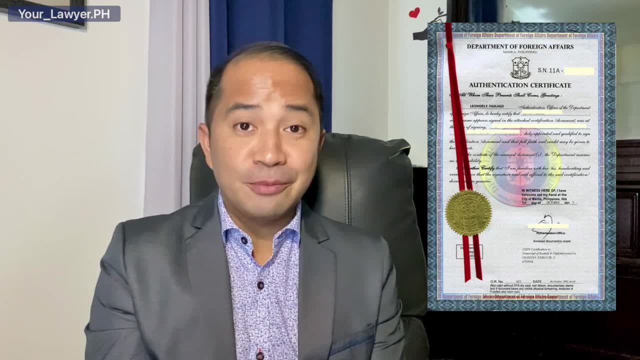 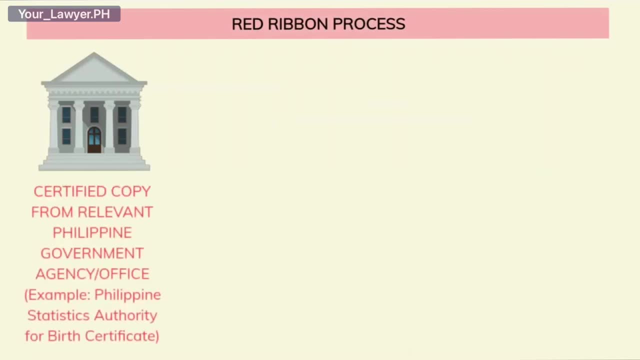 ang document na to sa konsulado ng bansa kung saan mo ito gagamitin. Tinatawag po itong legalization or consularization. The old Red Ribbon process starts by getting a certification from the relevant government agency or office and then getting authentication by the Philippine. 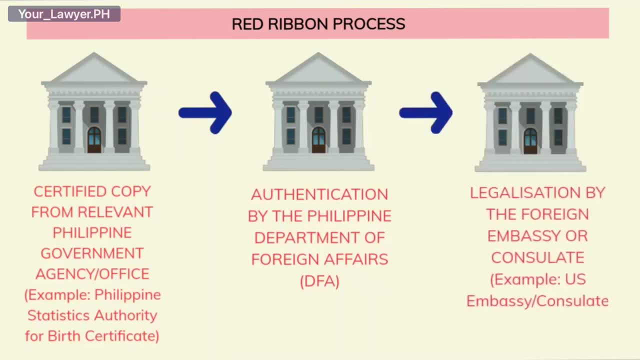 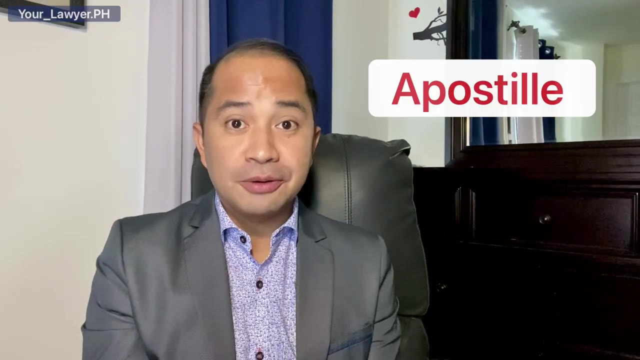 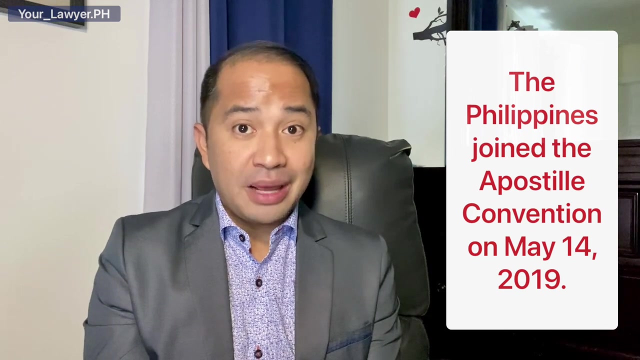 Department of Foreign Affairs. After the authentication by the Philippine Department of Foreign Affairs, you must then take your documents to the foreign country's embassy or consulate for legalization. But now you have a reason to rejoice, because the apostille has already replaced the Red Ribbon requirement when the Philippines joined the Hague Convention on Apostille on May. 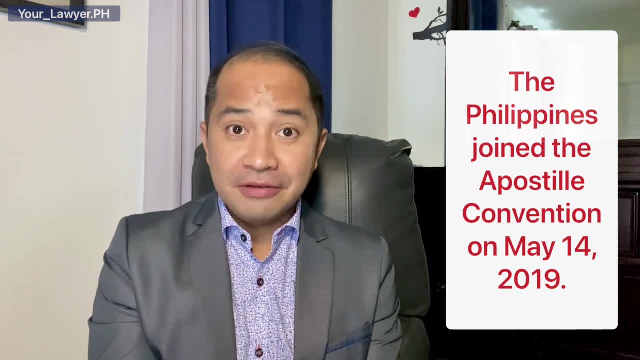 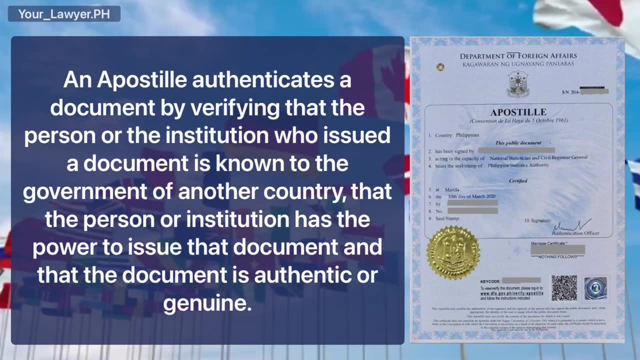 14, 2019.. Indeed, it was a sigh of relief, dahil mas simpli na po ang proseso. Ano ba ang apostille? Ang apostille ay nagpapatutuok kung ang isang dokumento ba ay tunay o authentic. Ito ay sa. 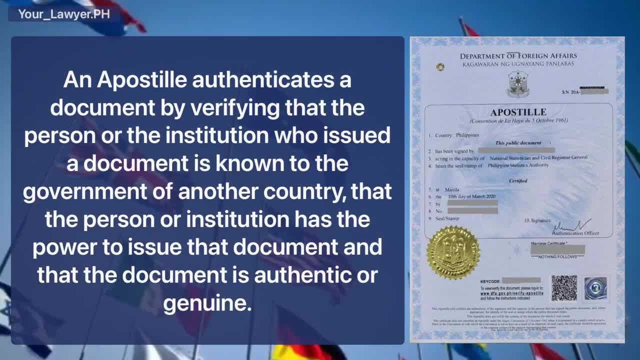 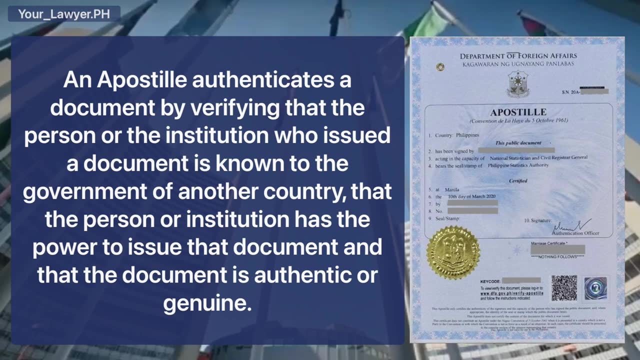 pamamagitan ng pagbibiripika o panglalaman. Ito ay sa pamamagitan ng pagbibiripika o panglalaman. Ang layunin ng apostille ay ang mapabilis ang proseso ng pag-authenticate ng mga dokumento. 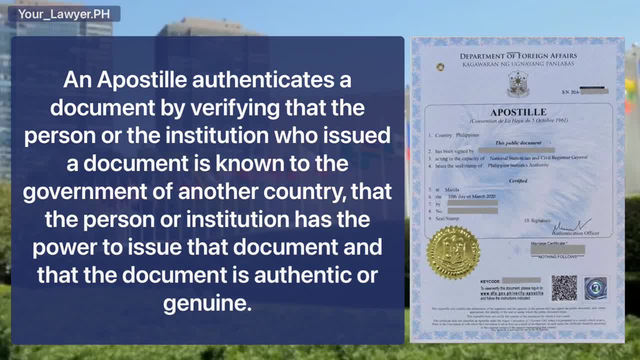 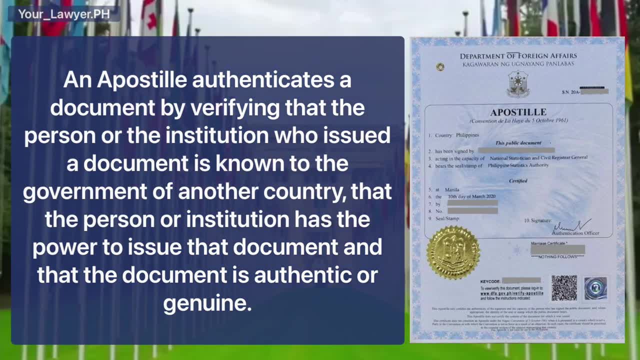 sa pamamagitan ng pagalis ng requirement ng legalization na dati ay ginagawa ng foreign embassy or consular agency. Ito ay sa pamamagitan ng pag-authenticate ng mga dokumento sa pamamagitan, In other words, tatanggapin sa ibang bansa ang dokumento as genuine on the basis of the 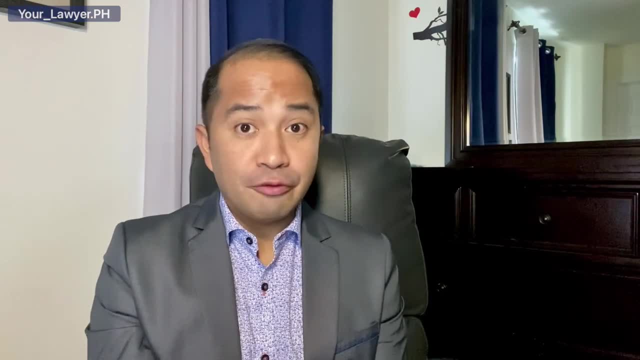 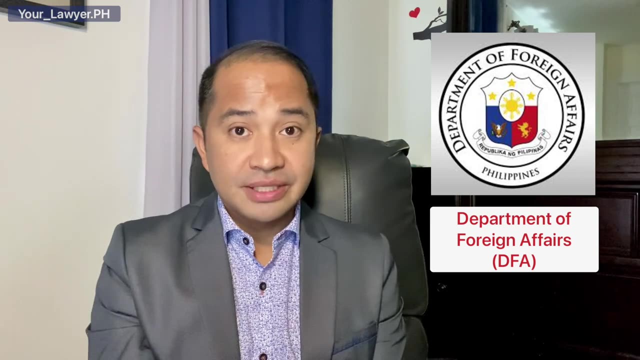 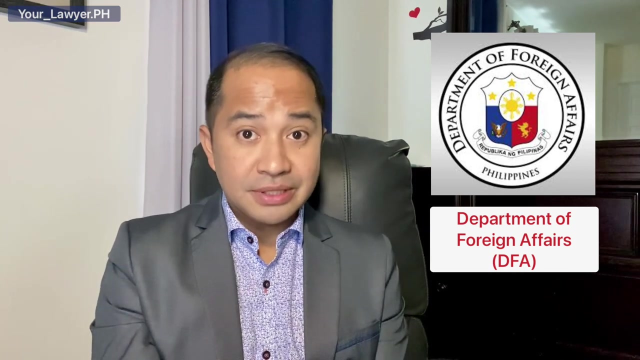 apostille In the Philippines tanging ang Department of Foreign Affairs o DFA, lamang po ang may authority o kapangyarihan na mag-apostillize ng mga documents At may mga identified na offices- ang DFA sa iba't ibang location sa Pilipinas na pwedeng mag-apostillize ng mga documents. 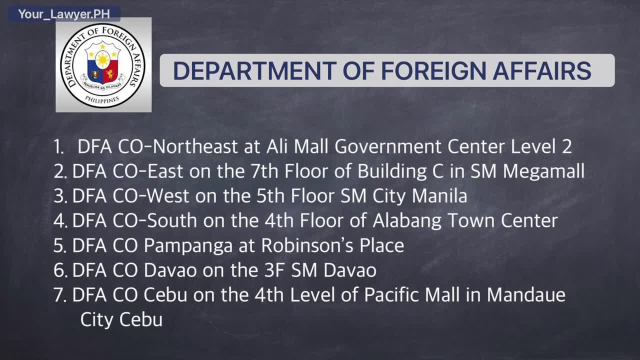 These are the DFA consular offices or satellite offices that offerocukulang postell deu misyo, kung ako na sigilan ulit saugo, kahit meron kayo Ang peles"As I have mentioned once your document. 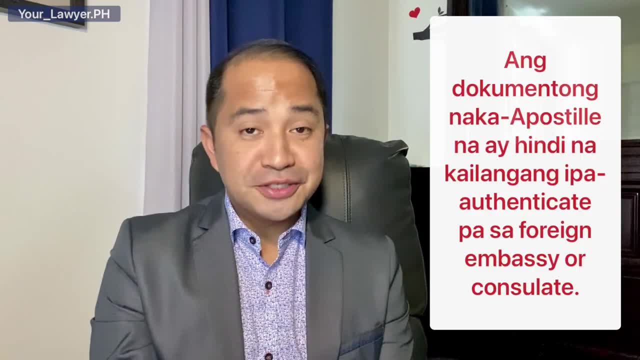 is already apostillized, there is no longer a need to haveyour document authenticated in the process called legalization or consularization by the foreign embassy or consulate". 地 braces kung iba't ipag- travaillkan sa mates atraves, mga apositeles atacle. 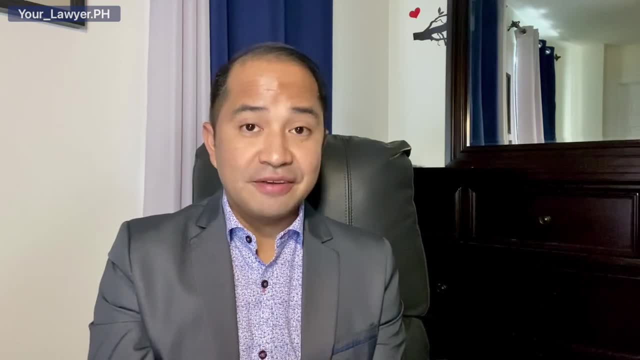 Kung ang special power of attorney mo ay naka-apostill na mula sa DFA ng Pilipinas, hindi mo na ito kailangang ipa-authenticate ng mga fees ng pag- размinal ng atale Cyong ang Akbar sa atale Brooke Gran Adam, who also in Catalonia na is pilot Ngaby P converte. 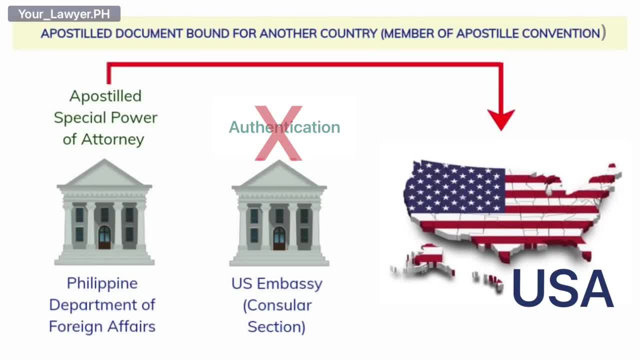 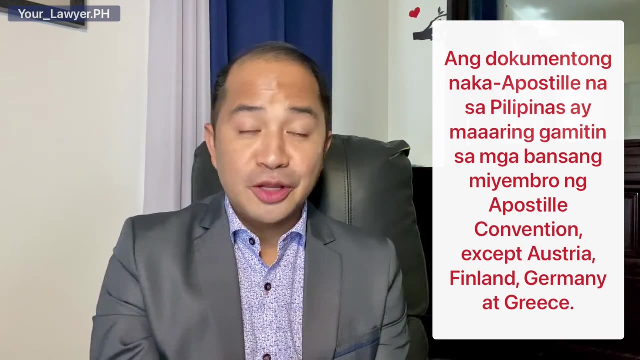 embassy or consulate upang magamit mo ito sa United States, sapat na ang apostille na basihan ng mga taga United States upang masabi na ang dokumento na ito ay authentic or genuine. Pwede mo rin gamitin ang dokumento na ito in United Kingdom, Australia, Japan, Spain. 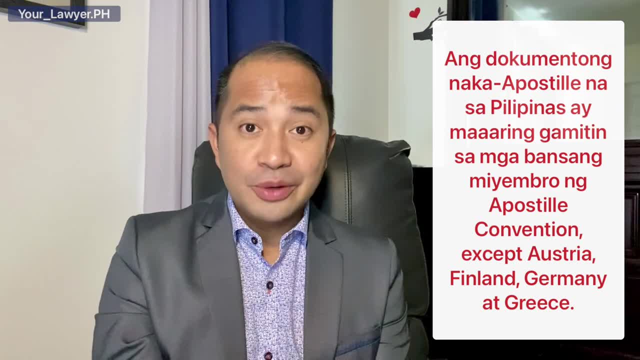 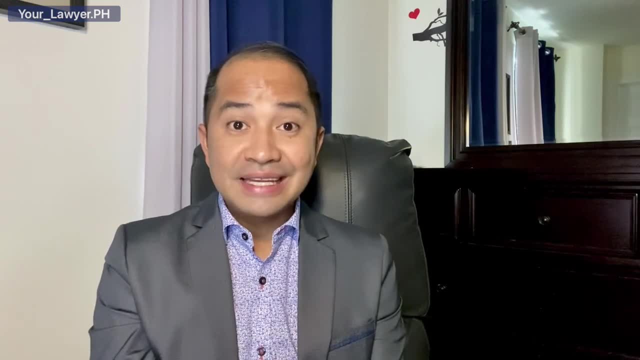 Norway, Denmark, Saudi Arabia or Italy, which are members of the Apostille Convention. It will not work, however, kung gagamitin mo ang dokumentong ito sa mga bansang hindi kasapin ng Apostille Convention o sa mga bansang nag-object o sumalungat sa pagsapin ng Pilipinas. 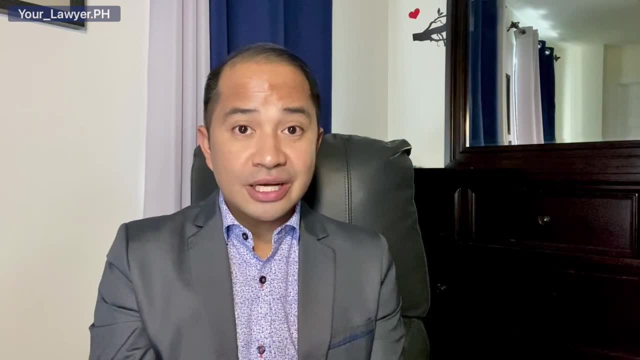 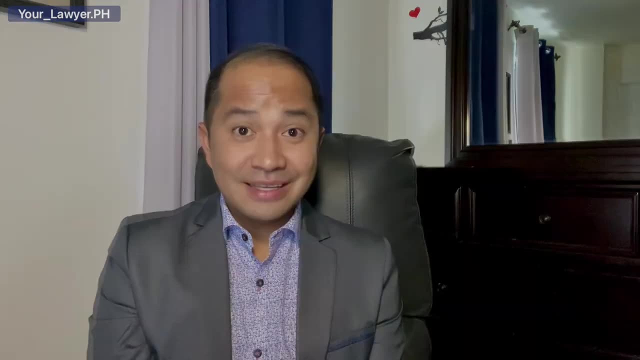 noon sa Apostille Convention. Ang mga bansang nag-object sa pagsali ng Pilipinas sa Apostille Convention ay ang Austria, Finland, Germany at Greece. In that case, kakailanganin mong ipa-legalize o ipa-authenticate ang dokumento sa imbahada. 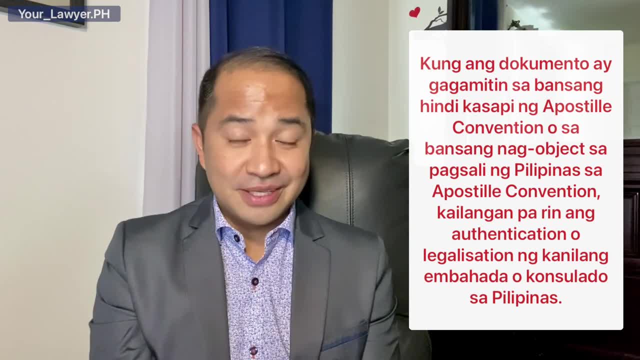 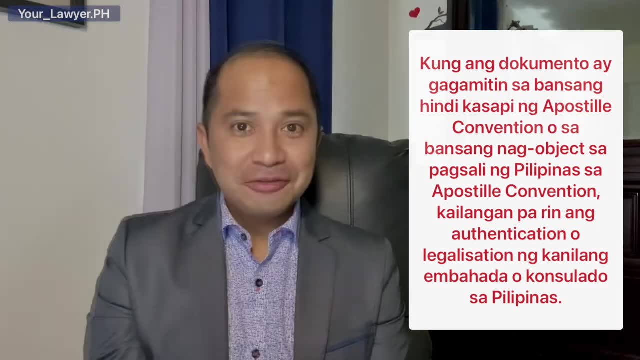 o konsulado ng bansang yun. Same as the old process. But before you do that, I suggest na alamin mo muna kung kailanganin mo muna, kung kailanganin ba talaga ang authentication for that document. 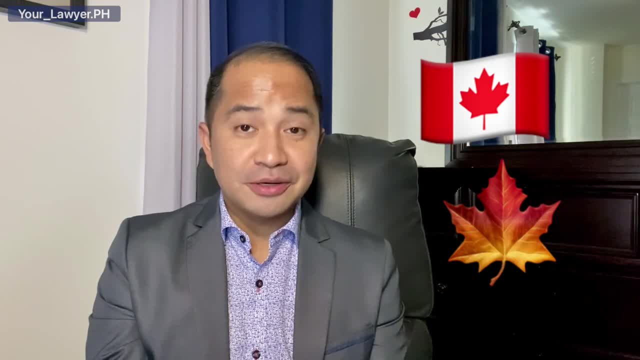 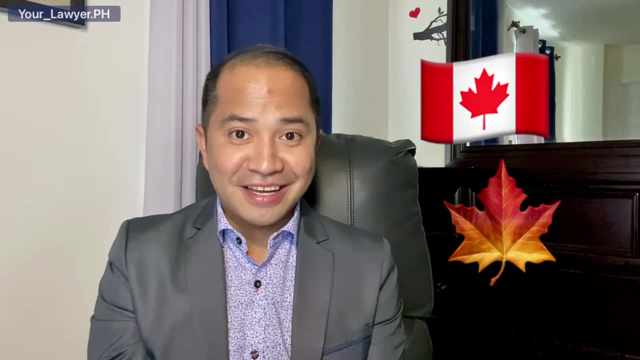 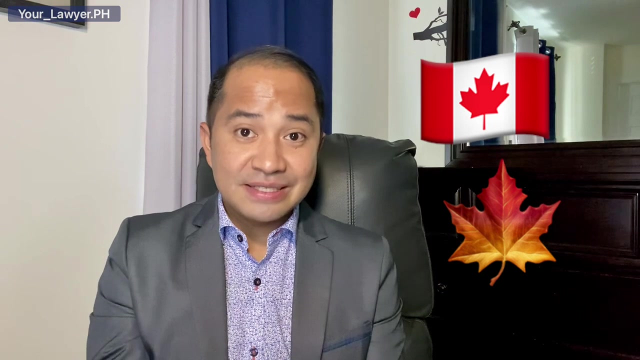 For example, Canada is not a member of the Apostille Convention because of the unique requirement when it comes to international agreements: Kailangan po kasi ang pagpayag ng mga provinces ng Canada. But I was surprised because when I applied for a driver's license in Canada, I presented 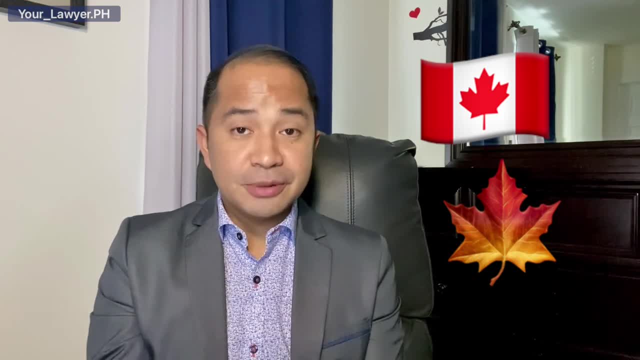 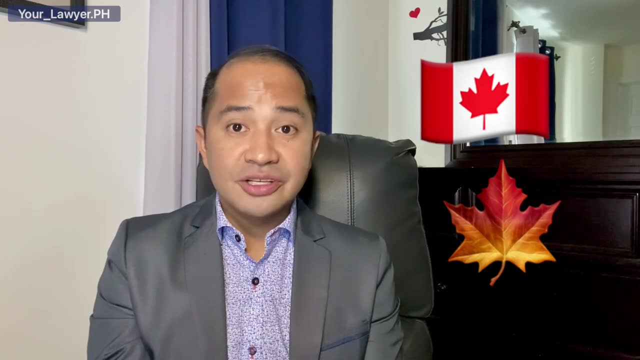 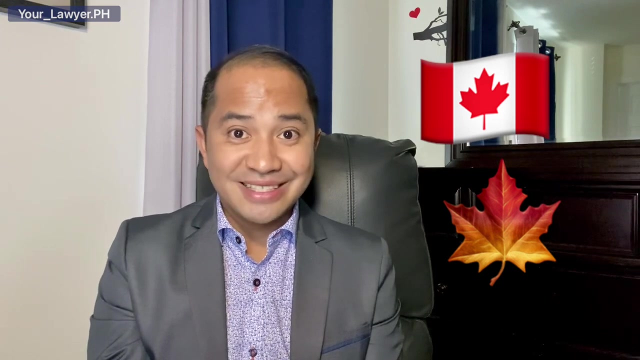 an Apostille certification from the Land Transportation Office in the Philippines and they simply required it to be authenticated. So I was authenticated by the Philippine consulate in Toronto and I was given the credits for the number of years that I was a licensed driver in the Philippines. 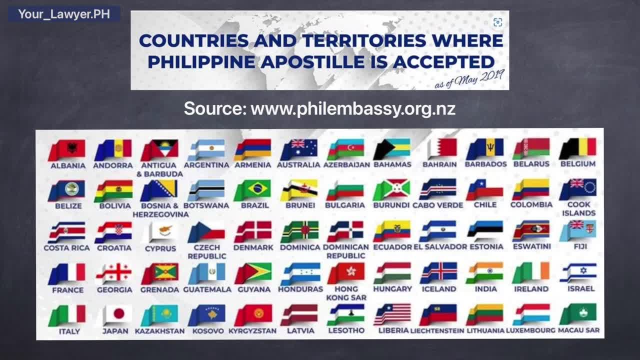 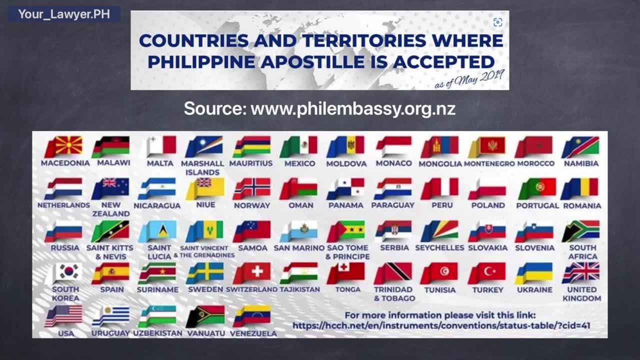 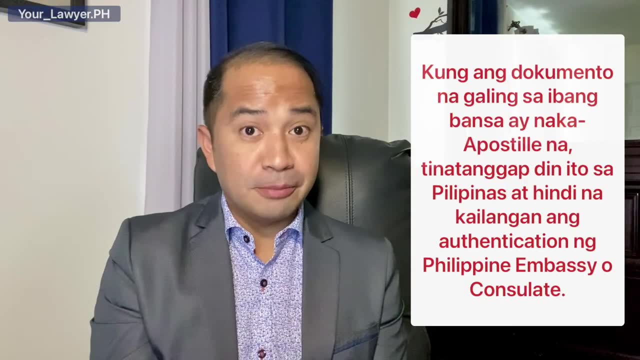 Ito naman po ang mga bansa at teritories na kasapi ng Apostille Convention. Please feel free to pause the video to find out if your country of residence ay kasapi po ng Apostille Convention, Kung ang dokumento naman po ay galing sa bansang kasapi ng Apostille Convention at gagamitin. 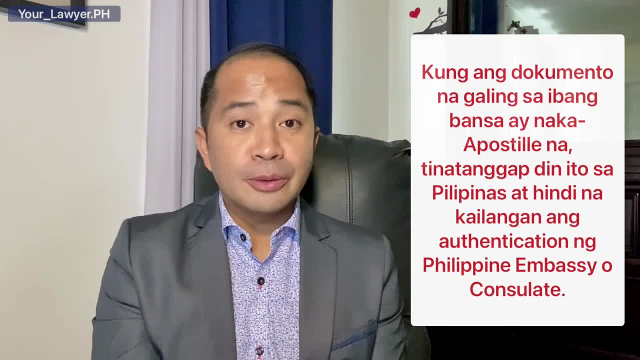 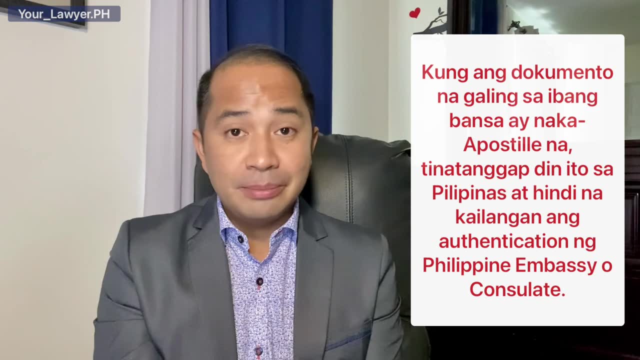 ito sa Pilipinas. The same rule applies: Kung ang dokumento po ay naka-Apostille na pwede na itong gamitin sa Pilipinas, at hindi nyo na po kailangang dalhin ito sa imbahada or konsolado ng Pilipinas upang ipa-legalize. 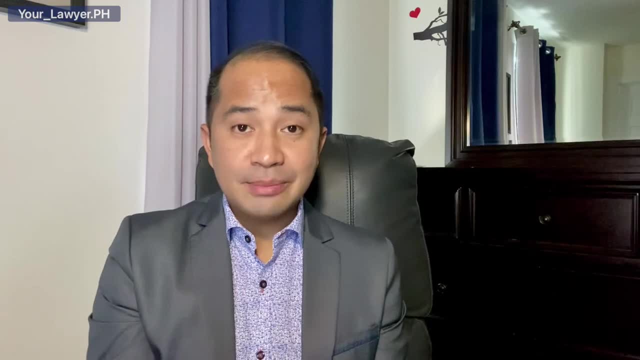 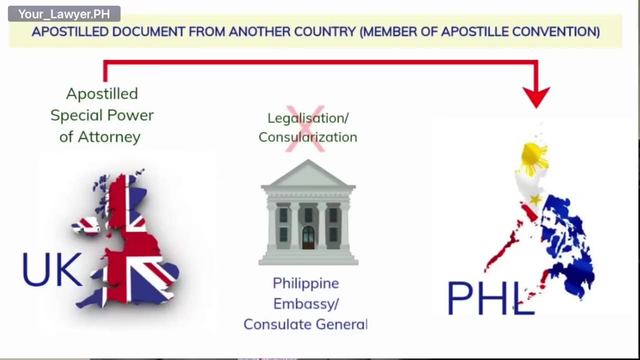 o ipa-consolarize Alimbawa, kung kayo po ay nasa bansang kasapi ng Apostille Convention at nais nyo pong magpadala ng Special Power of Attorney sa inyong representative sa Pilipinas para sa inyong transaction sa. 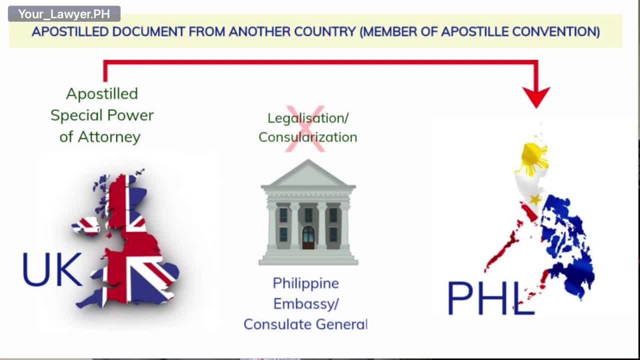 Pilipinas. sapat na po ang apostille. Hindi nyo na po kailangang ipa-legalize o ipa-consolarize ang documento. Ito ay naka-Apostille na. Kung ang dokumento po ay naka-Apostille na, pwede na itong gamitin sa Pilipinas at gagamitin. 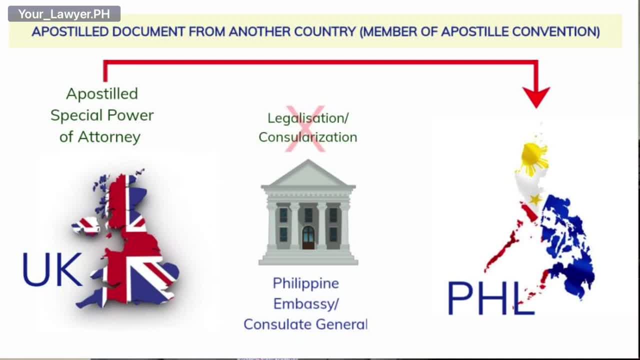 sa Pilipinas upang ipa-legalize o ipa-consolarize ang documento na ito sa Philippine Embassy or Consulate. Just be mindful lang po na magkakaiba rin po yung processes at requirements ng bawat bansa. 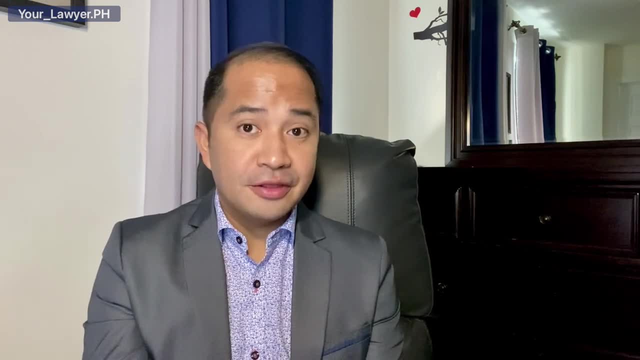 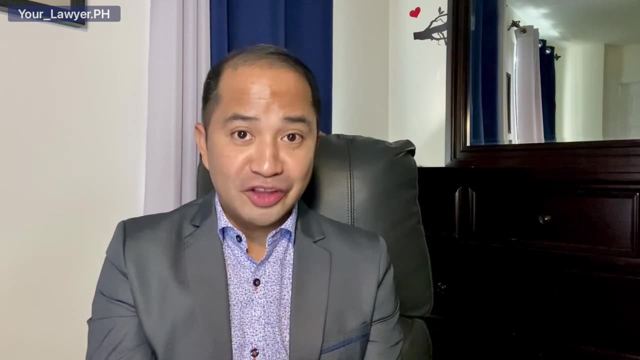 pagdating po sa pag-Apostille ng mga dokumento, and their respective laws may authorize certain persons or agencies na pwedeng mag-Apostille ng mga dokumento. Para naman po dun sa mga bansang hindi member ng Apostille Convention, ganun pa rin po yung. 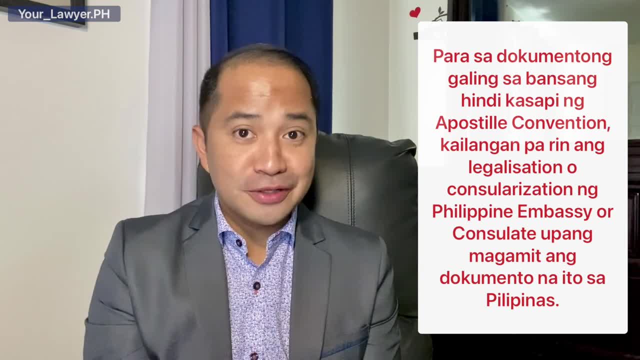 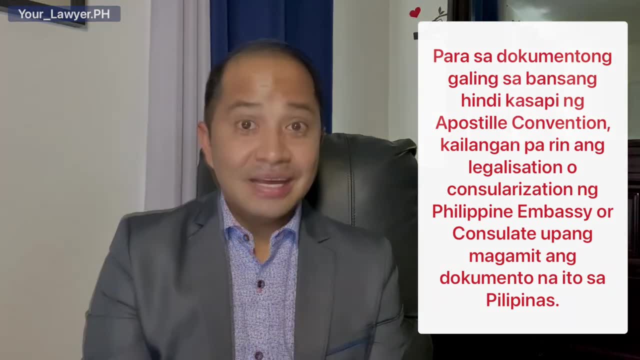 process Kailangang dumaan muna sa imbahada or konsolado. Ang mga dokumento ay magkakaiba rin sa Pilipinas for purposes of authentication, so that they can be honored or accepted in the Philippines. 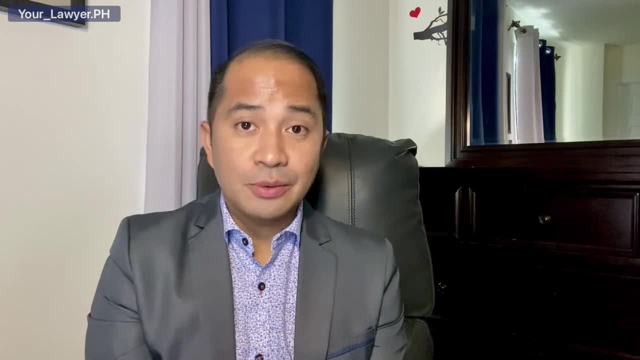 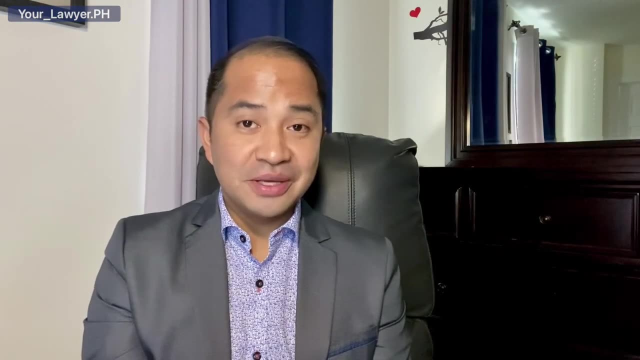 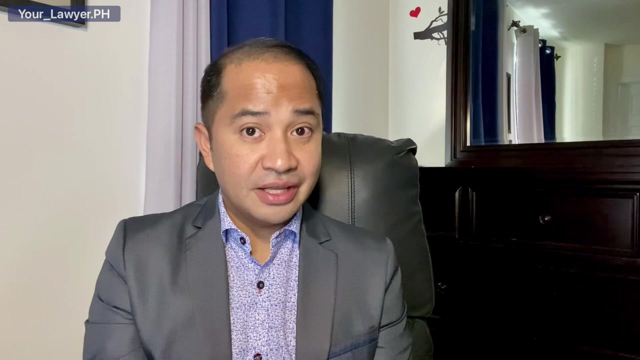 As to what documents can be apostilled or apostillized, I will put the link in the description box of this video. So just very quickly, what's the new process now in the Philippines? Say, for example, you want to submit a Philippine document abroad like a notarized affidavit. 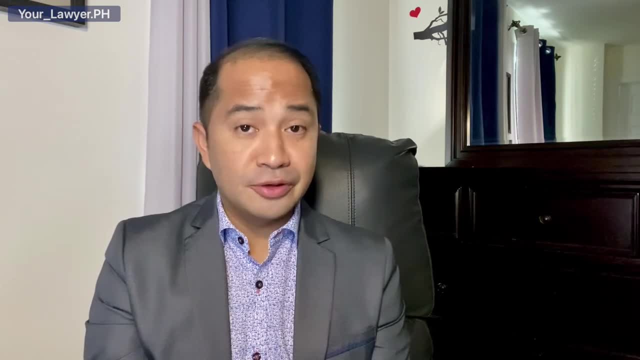 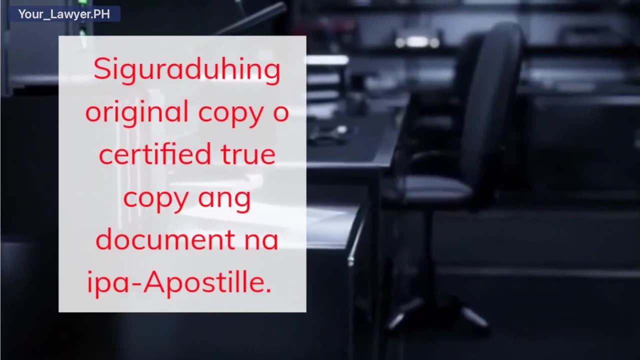 special power of attorney, NBI clearance or a certificate of no marriage. What is now the procedure? First, you need to have the original document at hand. If it is a birth certificate, kailangan ang kopyang galing sa Philippine Statistics Authority. 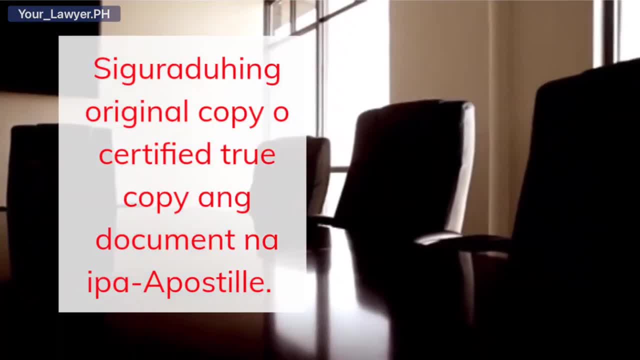 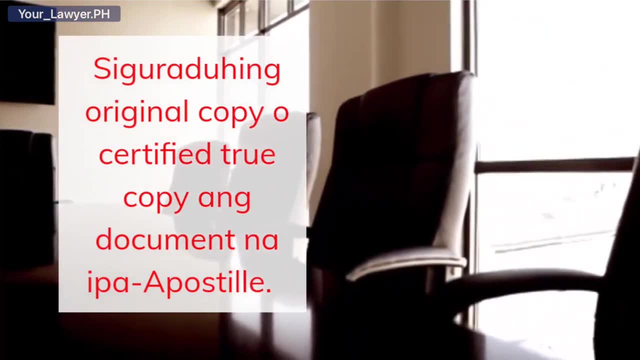 Kung certificate of driving experience dapat, galing ito sa main office ng Land Transportation Authority. Kung hindi original ang document, pwede naman ang certified through copy. Remember, hindi pwedeng ipa-Apostille ang photocopy or xerox copy. 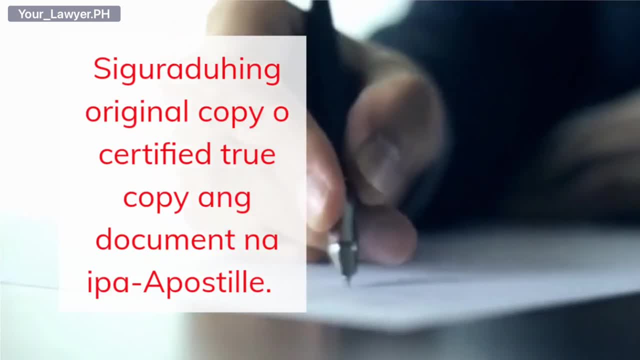 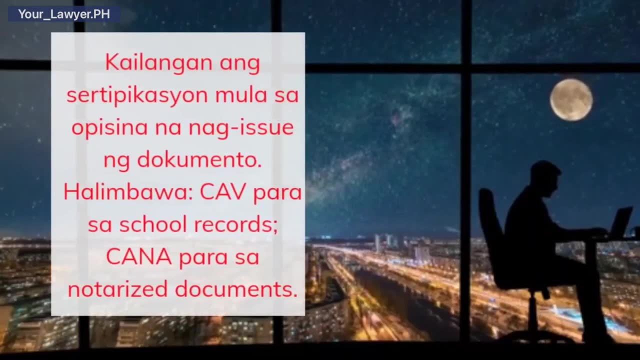 Ilalagay ko po sa description box ng video na ito Ang link para sa listahan ng mga dokumento na pwedeng ipa-Apostille. Second, that original document must be certified by the issuing office or agency. Halimbawa kung school records, ito dapat certified copy ito na inisyo ng eskwelahan. 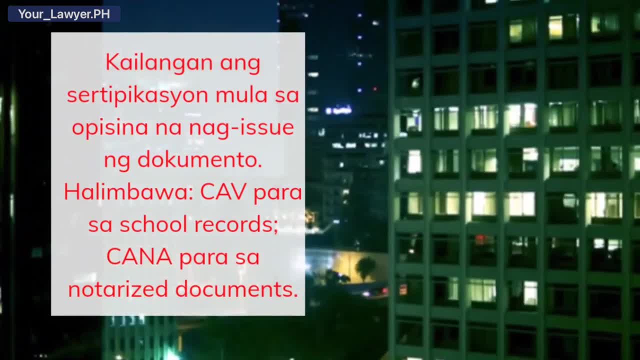 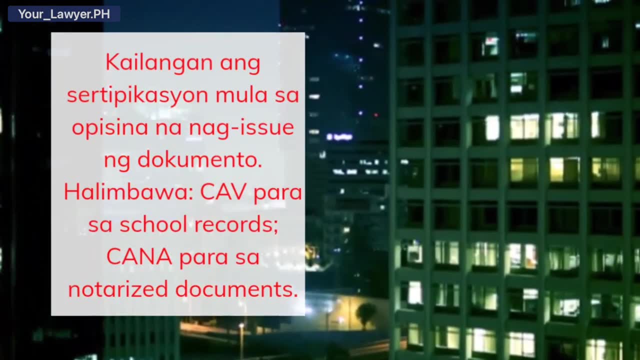 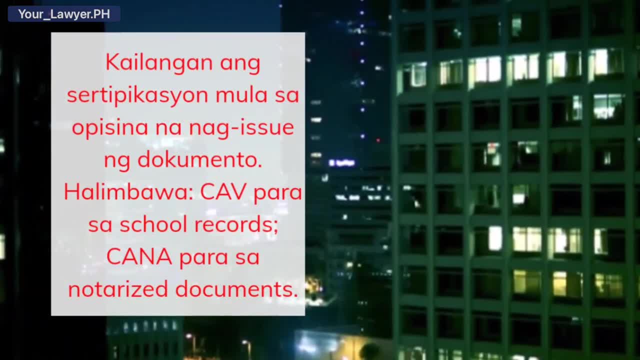 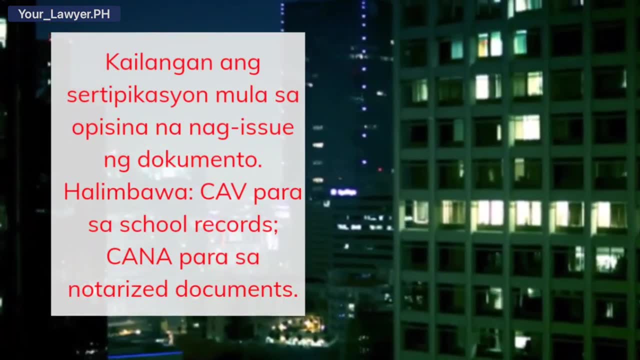 So ito ay isyat. So ito ay isyat At TESDA naman, para sa mga technical o vocational courses, Kung state colleges and universities for transcript of records and diploma certified through copy and certification, authentication and verification from the school, 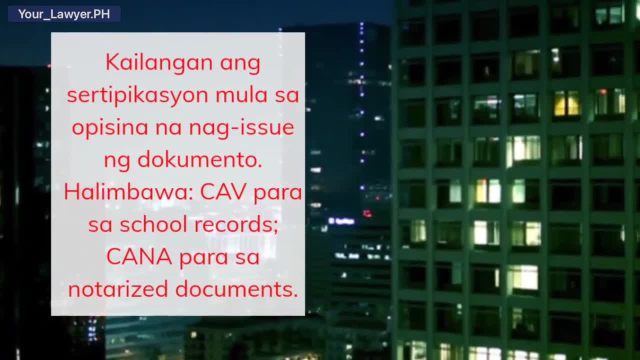 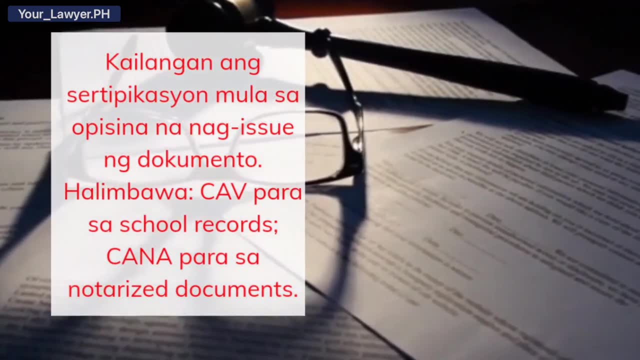 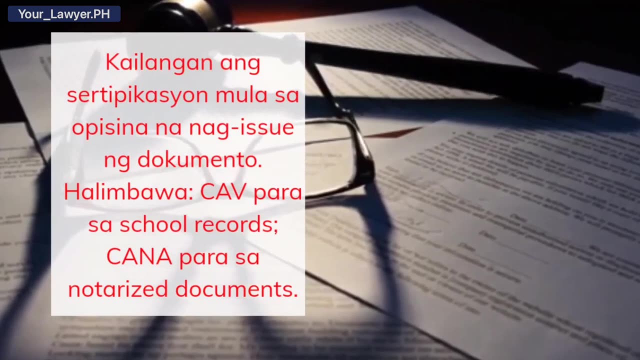 For notarized documents, katulad ng special power of attorney, affidavit o kontrata, dapat may kalagip itong CANA o Certificate of Authority for a Notarial Act signed by the executive judge or vice executive judge Or any office authorized signatories na galing sa regional trial court. 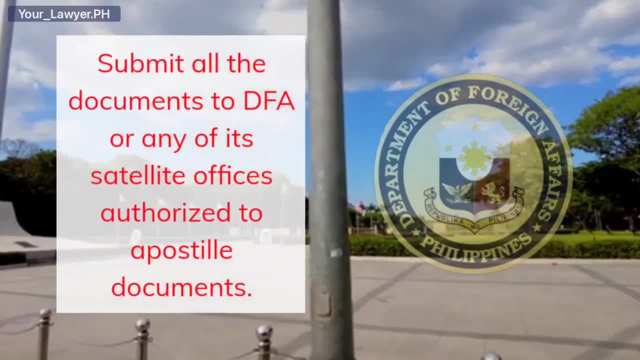 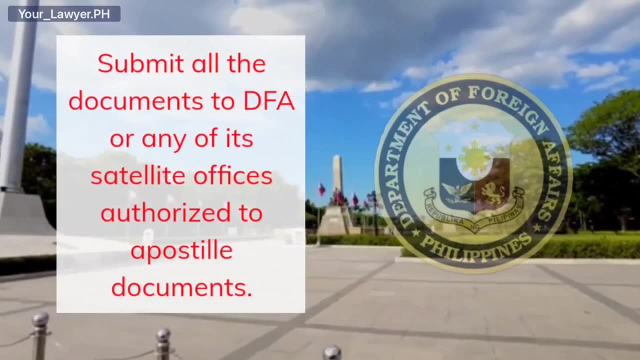 Kung kumpleto na ang mga dokumento, all you have to do is to submit the documents to the DFA or to any of its satellite offices na nabanggit ko kanina. As of now, I think required pa rin ang online appointment bago kayo pamunta sa kanilang. 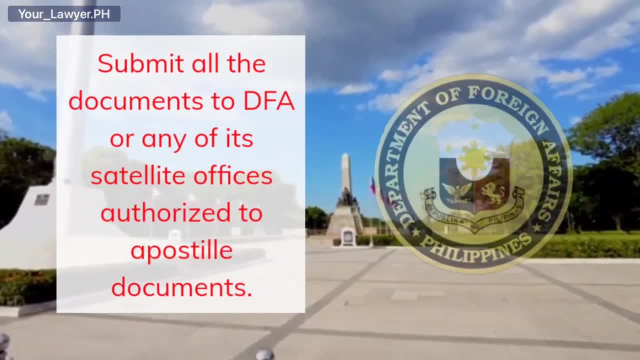 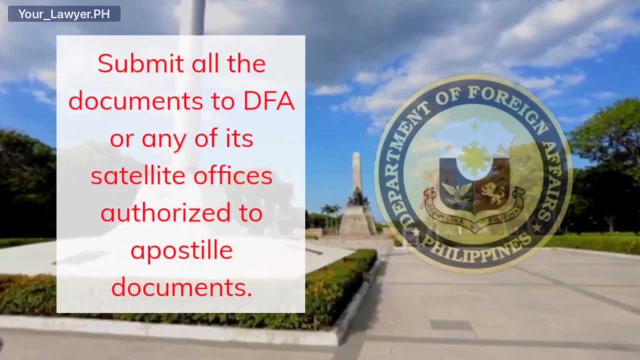 opisina. So kailangan nyong mag-book ng appointment online. I will put the link for online appointment in the description box of this video. You will be required to pay $100. For regular processing, at 200 pesos naman for express processing, which can be released. 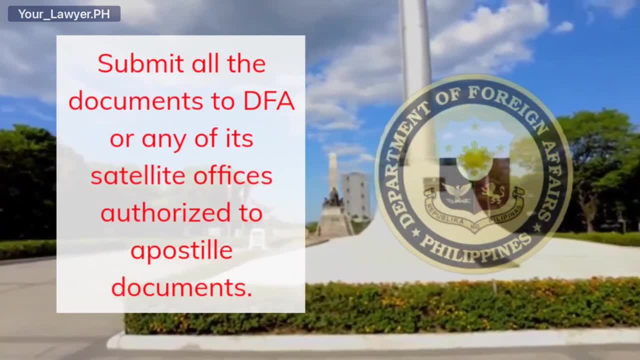 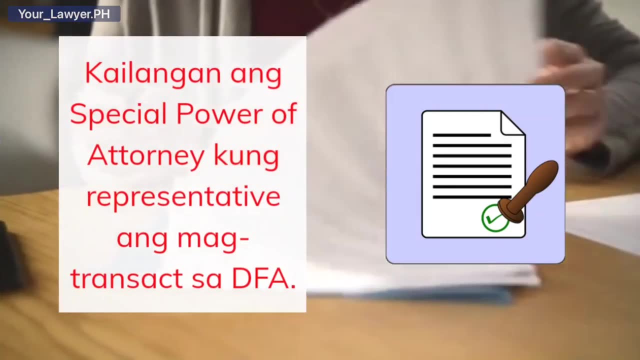 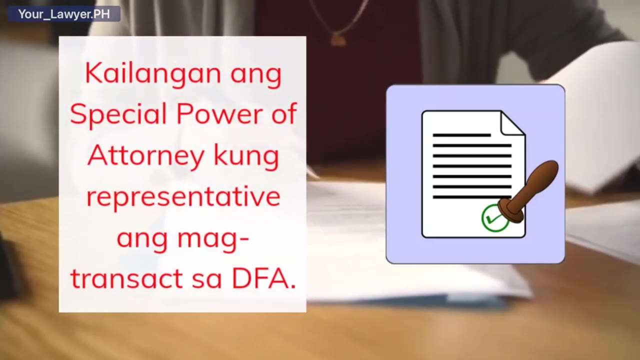 on the following day. Just check on the website of the DFA for possible changes. If you cannot process it personally, you can send an authorized representative to process and claim the documents on your behalf, provided that the representative presents the following Authorization letter from the owner and for minor applicants: 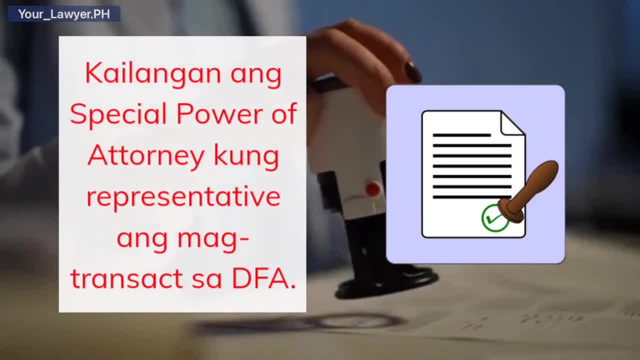 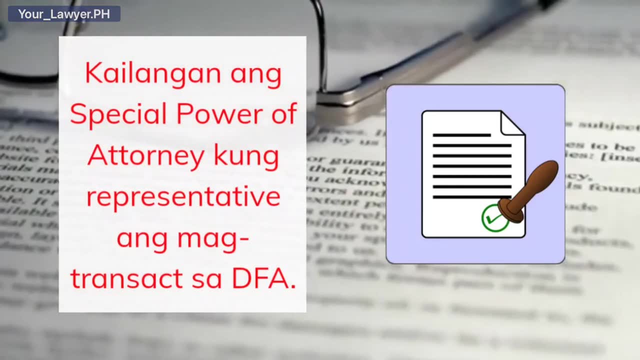 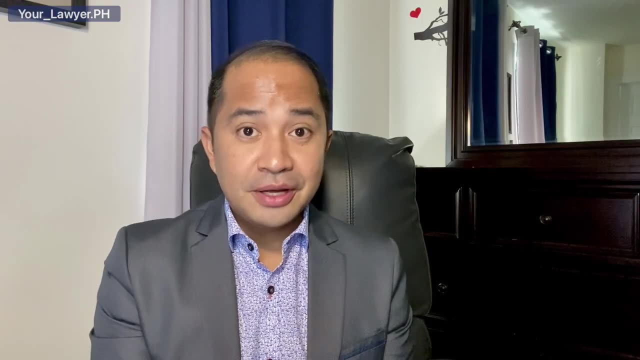 The power of attorney must be executed by the parent or parents. The photocopy of the owner's ID which bears his or her signature, The photocopy and original copy of the representative's ID, As I have mentioned earlier. once you already have the apostille document, you can use it. 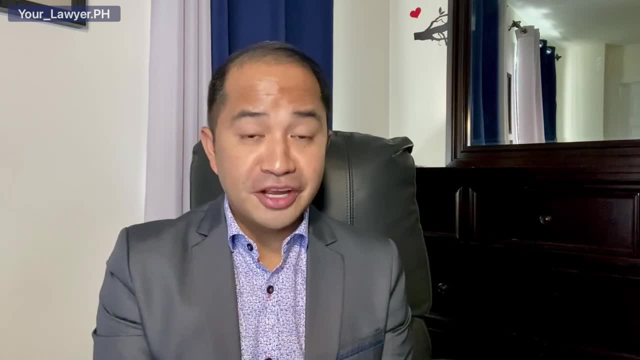 in any of the countries that are members of the apostille convention, except for Austria, Finland, Germany and Greece. This is what makes it different from Red Ribbon, Kasi ang doko ko si red ribbon. Ang dokumento na na Red Ribbon na ay pwedeng gamitin lamang sa bansa ng embassy or consulate. 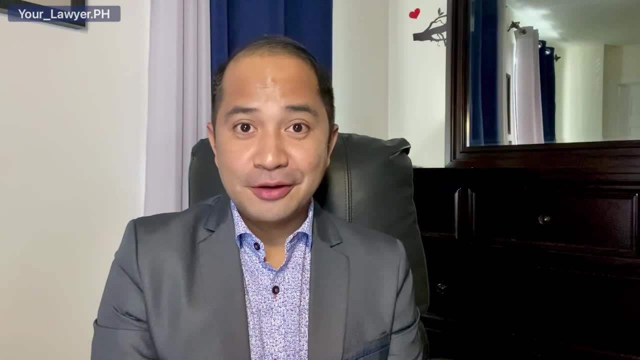 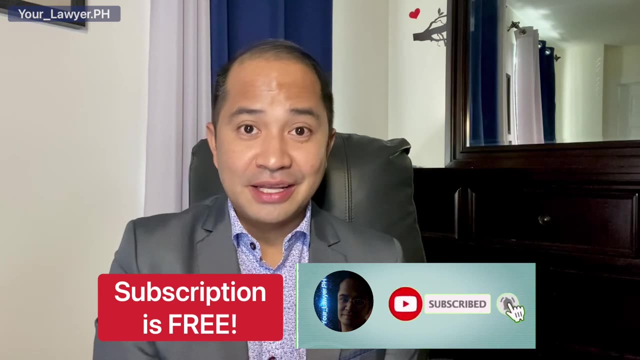 na nag-authenticate ng document. I hope that you have learned something from this video. Please don't forget to subscribe to this channel if you haven't done it yet, and hit that notification bell icon so that you will get notified of our future videos. 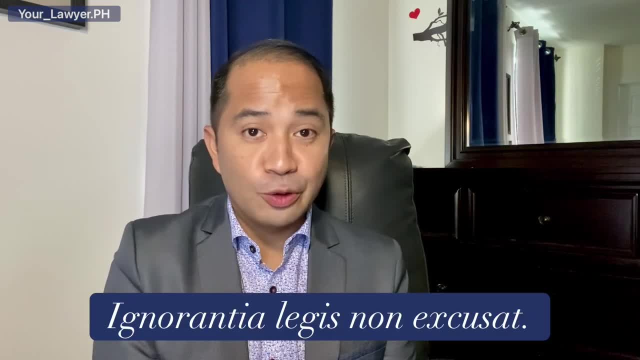 Always remember: ignorance of the law excuses no one from compliance therewith. I will see you in my next video. Ingat po kayo. Bye for now.